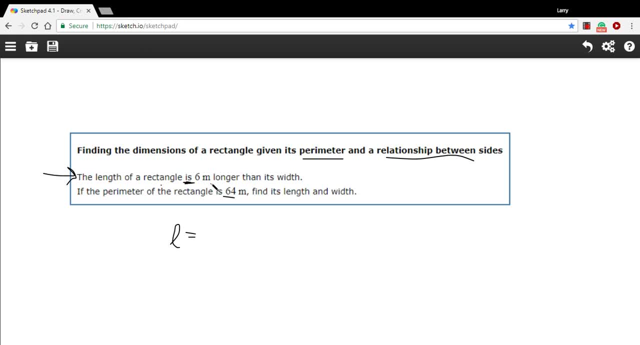 equal sign. and then this part we need to translate: six meters longer than its width. Well, the width of a rectangle is W. To be six meters longer than W, you would just add six meters. So this is the equation from this sentence, and this is important because 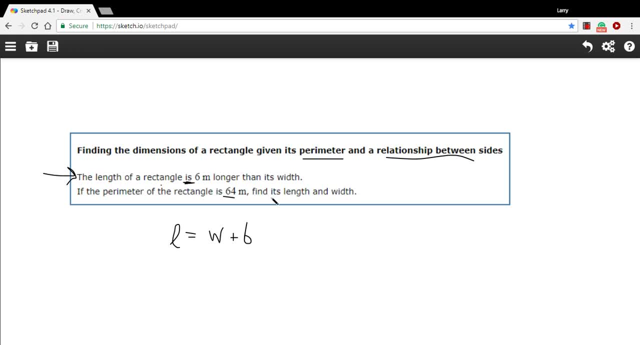 we're going to use this equation when we write out the equation for a perimeter. Now, the perimeter of a rectangle is the width plus the width plus the length plus the length, and so we could write this as width plus width plus, and now I could put an L plus L here, but we know L equals W plus six, so I'm just going to. 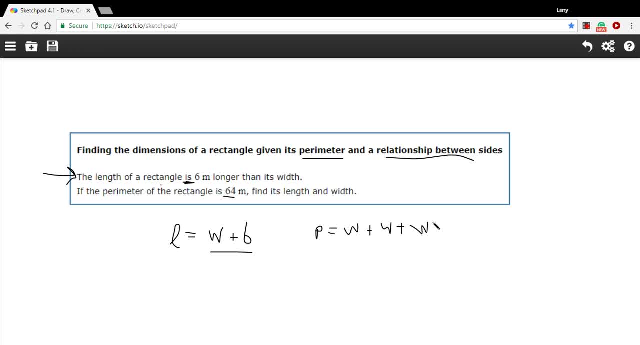 put in two of those. so W plus 6, that's a length. plus W plus 6, that's another length. So now we have the perimeter here, Two widths, two lengths, and we know the perimeter equals 64, so we can put that in for P. Let me bring all this down. 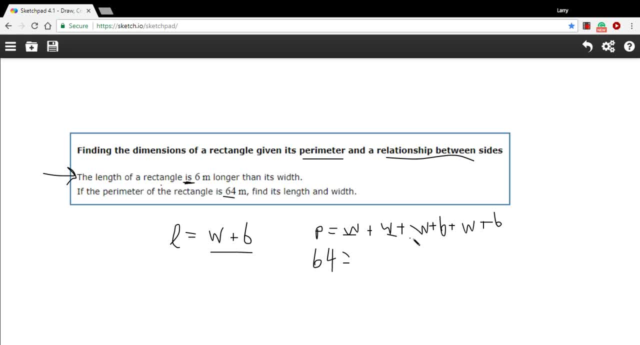 after I simplify it, Let's combine like terms. we have WWWW, that's four W's, and we have 6 and 6,, that's 12.. Now we just need to do a little bit of algebra to solve for w. I'm going to start by subtracting 12 so we can get that w term alone. 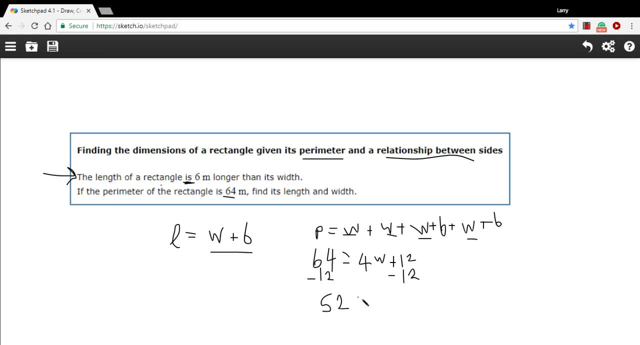 So this would be 52 here and 4w, And then we just need to divide both sides by 4 to get the w totally alone, And 52 divided by 4 is 13. So w equals 13. Not quite done yet, though. 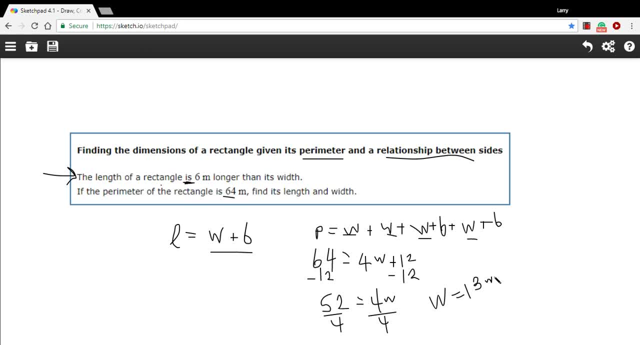 And let's see This was meters. Remember we said the length is w plus 6.. So I'm just going to take 13 plus 6.. So our length is 19 meters. So that is a little bit of work with finding the dimensions of a rectangle. 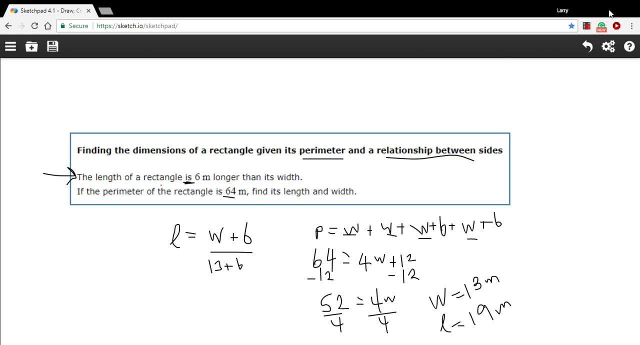 when they give you a perimeter and just a relationship between the sides. It should look like this For our reflection: if we want to look at the side of the rectangle, we're going to look at the side of the rectangle And what we're going to do is find the size of the rectangle and then we're going. to apply the Она to this side of it. And now we just need to replace the bottom and top of the rectangle. So I'm just going to take and replace the bottom of the rectangle with the inside. So I take the top of the rectangle and I replace the inside with the inside. And the next problem is the center. the center is going to come down. This one is going to be a little bit of a long, but it's going to have to be a little bit of a long time. That's about it.